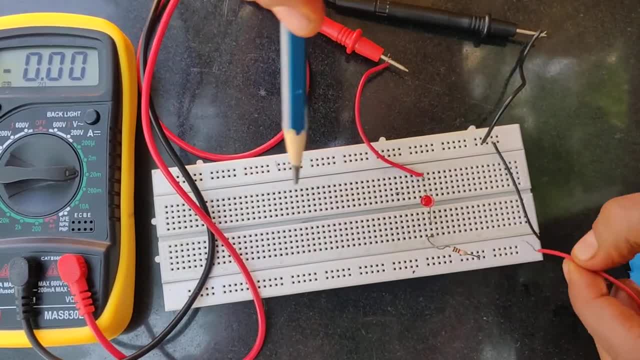 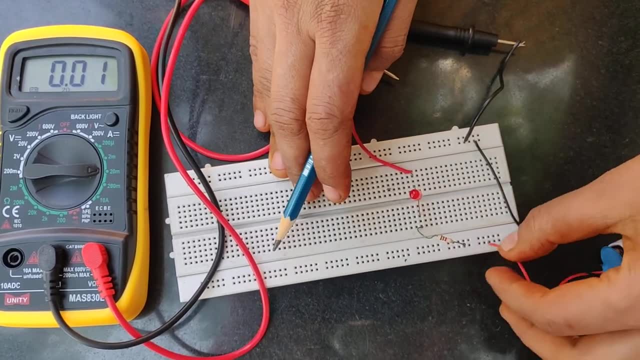 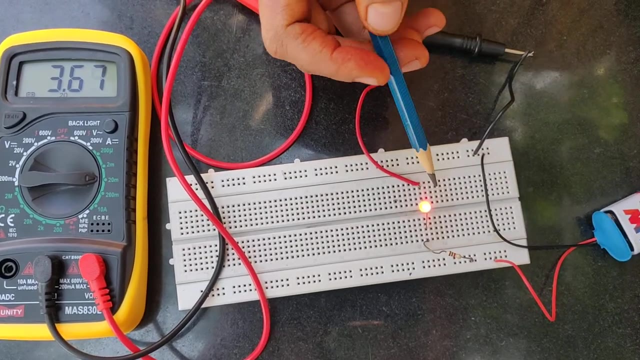 meter, just to see the current measurement. So I am connecting this battery positive, battery positive- to resistor. Yes, now you can see LED has started giving us output light and, as well as, we are going to connect this battery positive to resistor. So we are going to 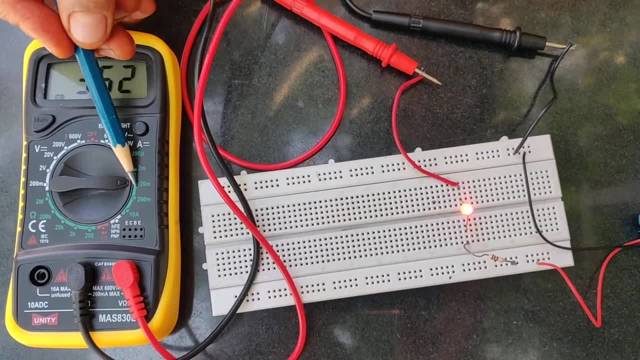 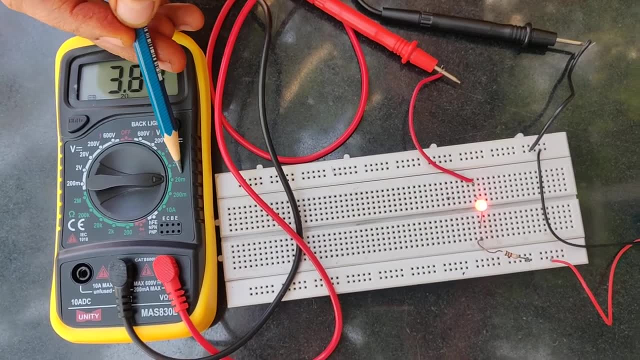 connect this battery positive to resistor. Yes, now you can see. LED has started giving us output light. you can see the current 3.54 milli ampere current is flowing through the circuit. So this is how we can measure current and we have chosen the appropriate range for current. 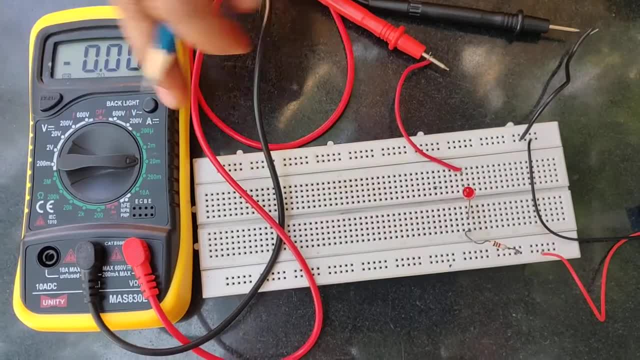 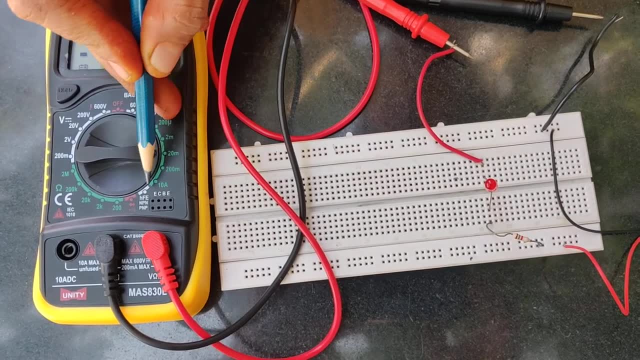 Okay, so how I have chosen the range. let us see that the maximum appropriate available for us that is 200 milli ampere. This is very, very high, So we are not going to consider this 10 ampere current range. So for us, this 200 milli ampere current range is going to be 0.6 milli ampere current range. 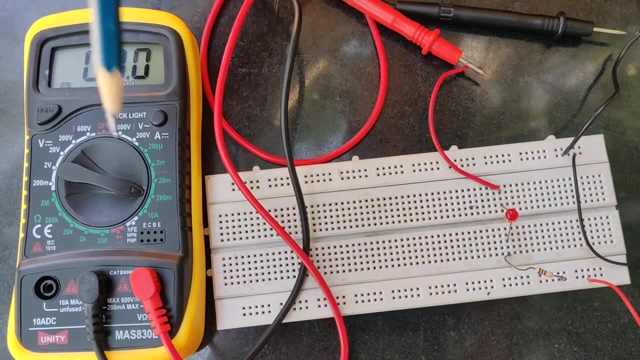 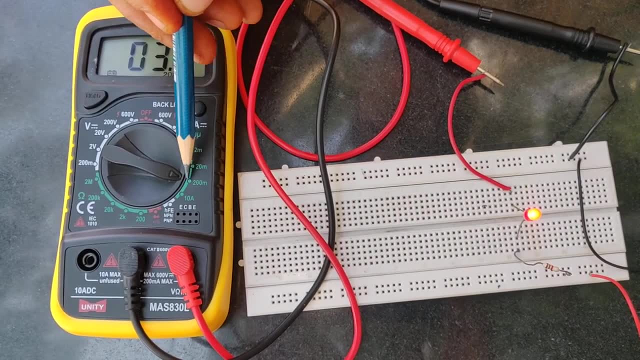 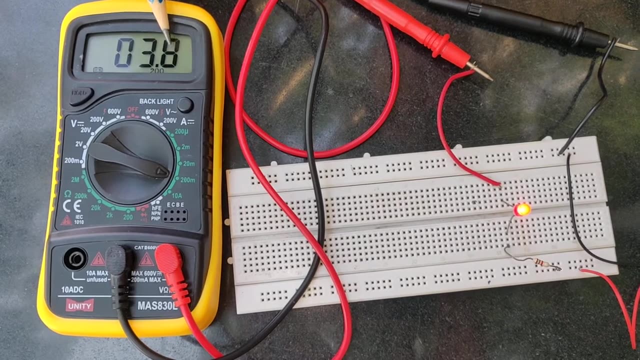 milliampere range is sufficient. fine, first of all, i have connected it and i have chosen the range. first of all, we have chosen the range, 200 milliampere, and you can see the display that it shows 3.8 milliampere. this is the maximum current flowing in the circuit, so we can. 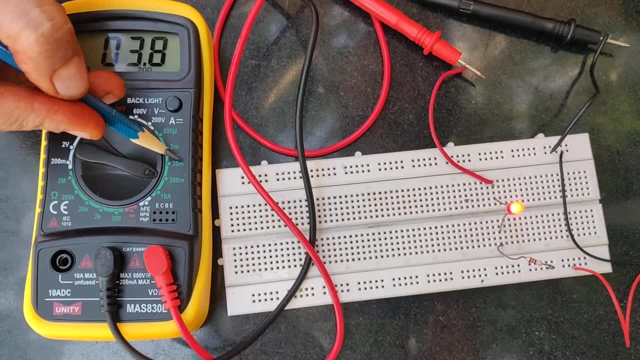 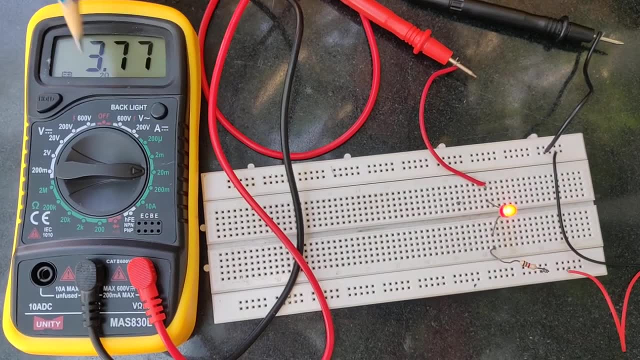 a step go down. that is 20 milliampere. we know it very well. 3.8 milliampere will definitely show us the value in 20 milliampere. this is how we can get the precise result. so for that we have. 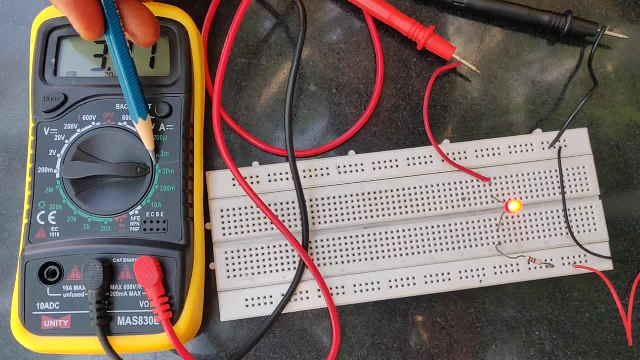 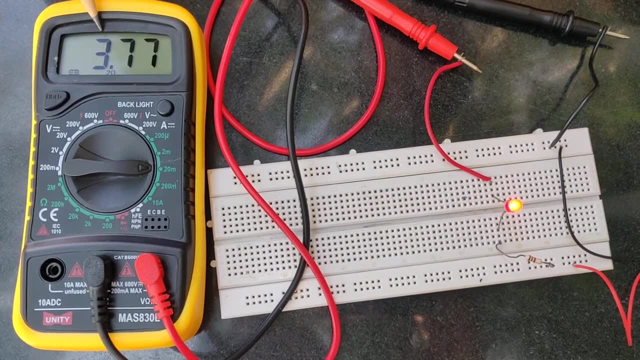 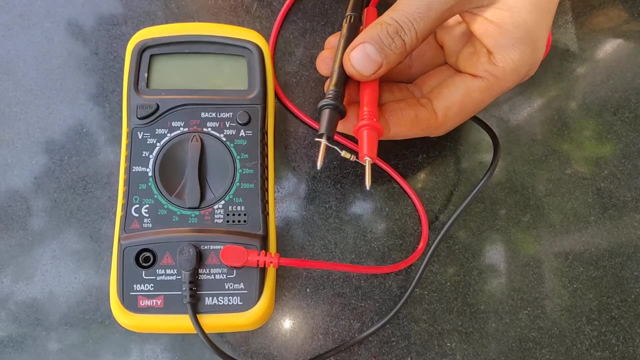 to always start from higher to lower. when you are interested to measure current, when you are interested in current measurement, right? so this is the precise result: 3.77 milliampere current flows in a given circuit. let us see the resistance measurement of a given. 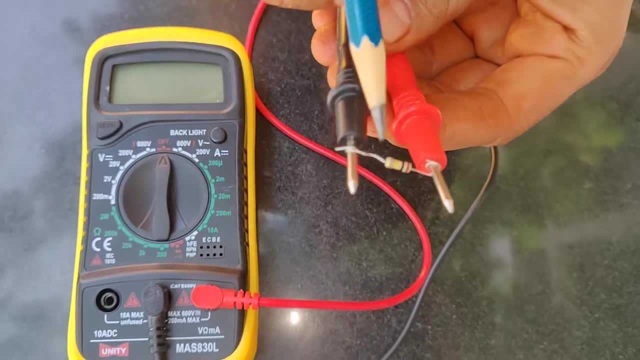 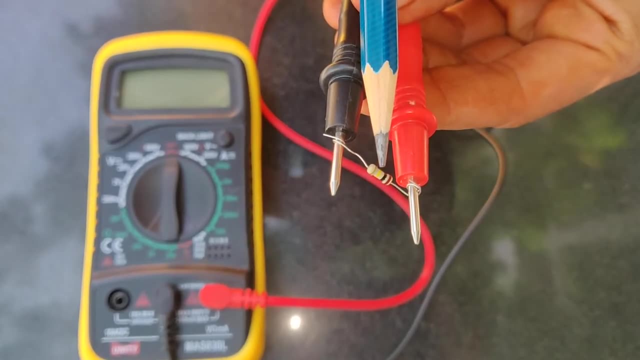 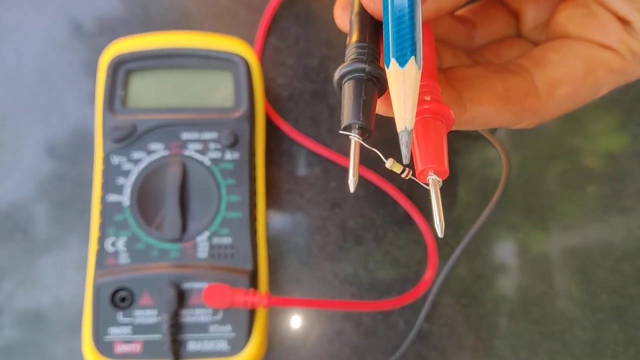 carbon pressure color code- fixed resistor. fine, so you can observe that the color band is given on the resistor: brown, black and yellow and the last one is for tolerance. so, as per theoretical value, we are having 1, 0 into 10 to the power 4. now let us see: are we getting the same value through?